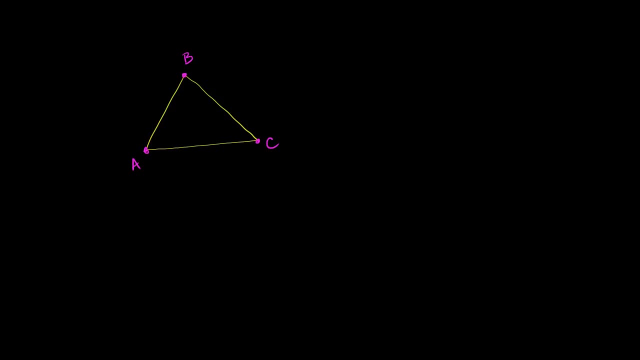 to draw an angle bisector for this angle up here, And we could have done it with any of the three angles, but I'll just do this one. It'll make our proof a little bit easier. So I'm just going to bisect this angle. angle ABC. 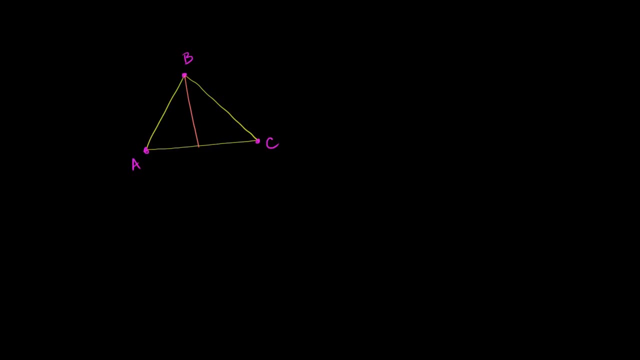 So let's just say that that's the angle bisector of angle ABC, And so this angle right over here is equal to this angle right over here. And let me call this point down here. let me call it point D: The angle bisector theorem tells us: 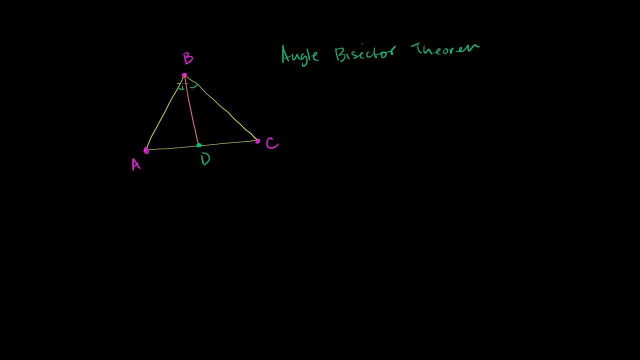 that the ratio between the sides that aren't this bisector. So when I put this angle bisector here, it created two smaller triangles out of that larger one. The angle bisector theorem tells us the ratios between the other sides, that of these two triangles that we've now created. 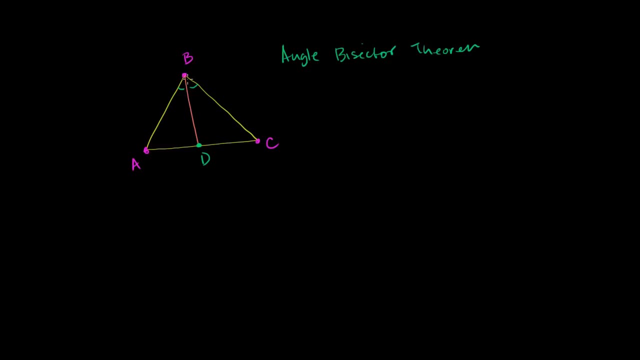 are going to be the same. So it tells us that the ratio of AB to AD is going to be equal to the ratio of BC to you could say CD. So the ratio of, I'll color code it the ratio of that. 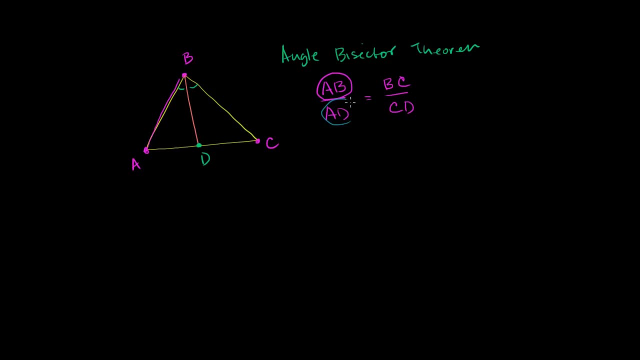 which is this To This, To this, Is going to be equal to the ratio of this, which is that to this, right over here, to CD, which is that over here. So it's kind of once you see the ratio of that to that. 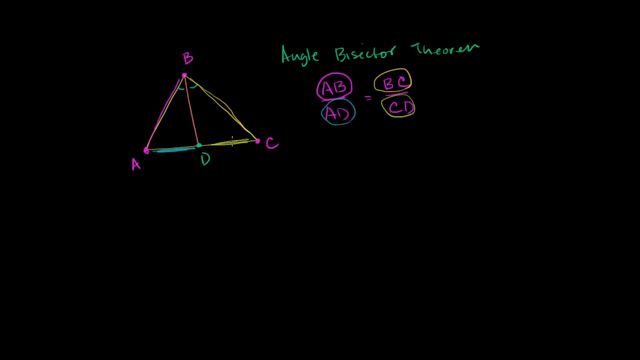 it's going to be the same as the ratio of that to that. So that's kind of a cool result. But you can't just accept it on faith because it's a cool result. You want to prove it to ourselves And so you could imagine right over here. 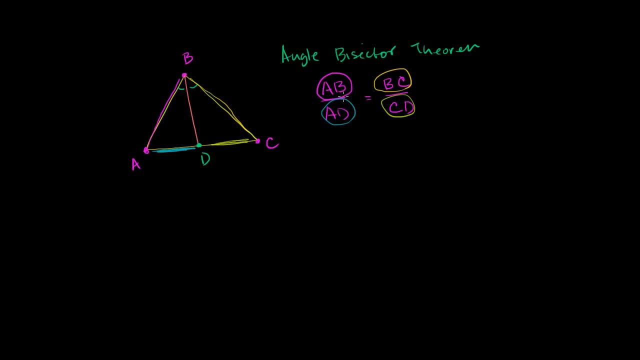 we have some ratios set up, So we're going to prove it using similar triangles And, unfortunate for us, these two triangles right here aren't necessarily similar. We know that these two angles are congruent to each other, but we don't know whether this angle is. 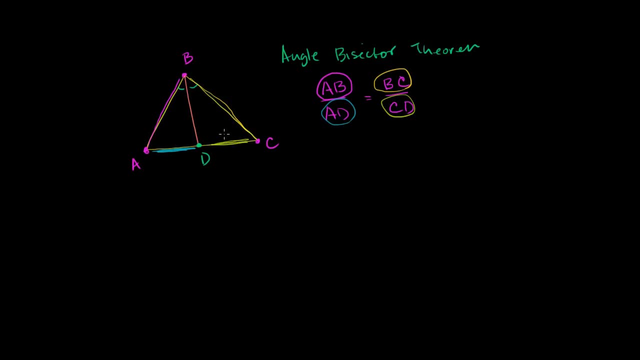 equal to that angle or that angle? We don't know. We can't make any statements like that. So in order to actually set up this type of a statement, we'll have to construct maybe another triangle that will be similar to one of these right over here. 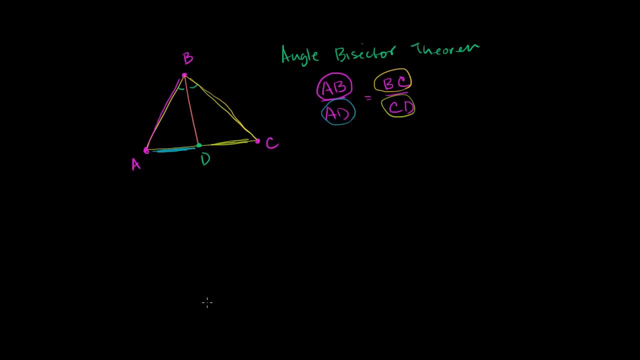 And one way to do it would be to draw another line. And this is a bit of this proof. wasn't there? It wasn't obvious to me the first time that I thought about it, So don't worry if it's not obvious to you. 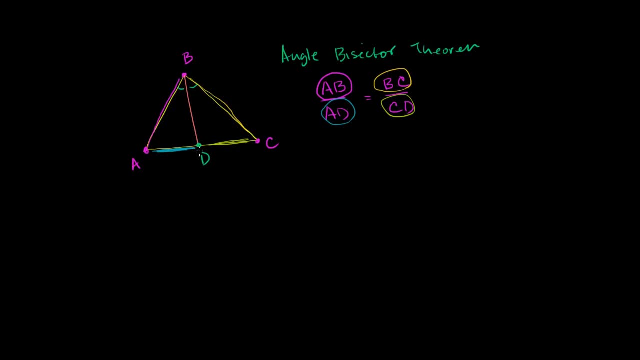 Is that? what happens is if we can continue this bisector, this angle bisector right over here. So let's just continue it. It just keeps going on and on and on And let's also. maybe we can construct a similar triangle to this triangle over here if we draw a line, that's. 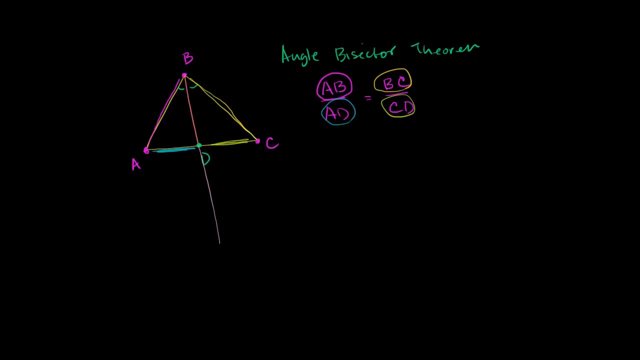 parallel to AB down here. So let's try to do that. So I'm just going to say you could always find if C is not on AB, you can always find a point that goes down, It goes through our line, that goes through C. 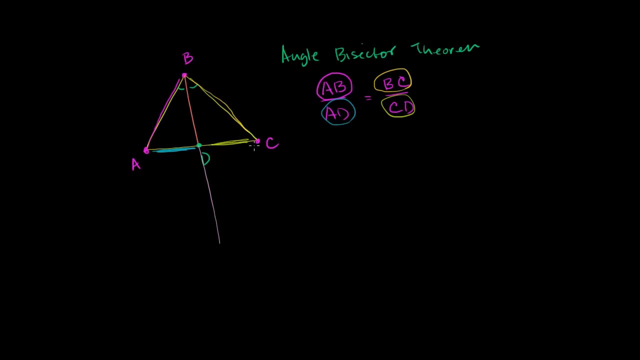 that is parallel to AB. So let's just, by definition, let's just create another line right over here And let's say: and let's call this point right over here: F, And let's just pick this line in such a way. 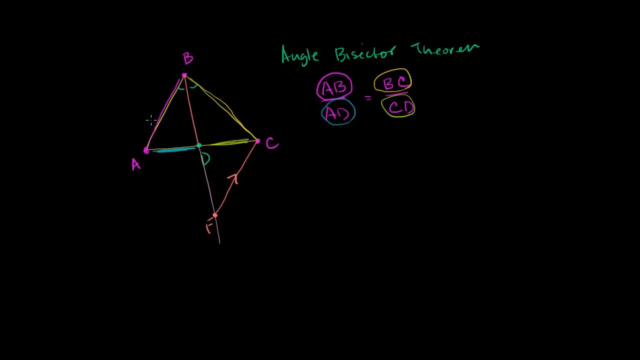 that FC is parallel to AB. So this is parallel to that right over there. So FC is parallel to AB And we could just construct it that way. And now we have some interesting things And we did it that way So that we can make these two triangles. 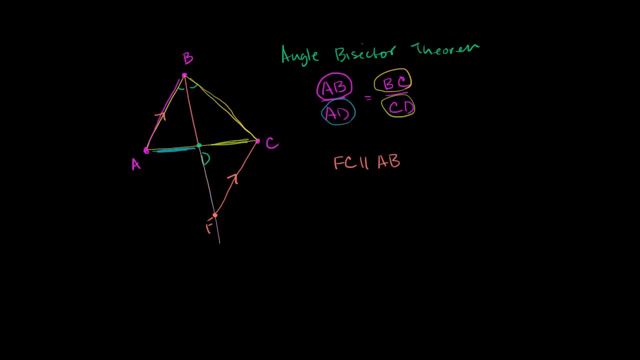 be similar to each other. So let's see that, Let's see what happens. So, before we even think about similarity, let's think about what some of the angles or what we know about some of the angles here. We know that we have alternate interior angles. 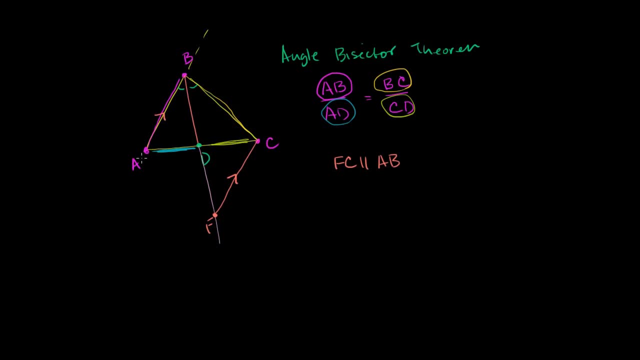 So just think about these two parallel lines. So I could imagine AB keeps going like that, FC keeps going like that And line BD right here is a transversal. Then whatever this angle is, this angle is going to be as well. 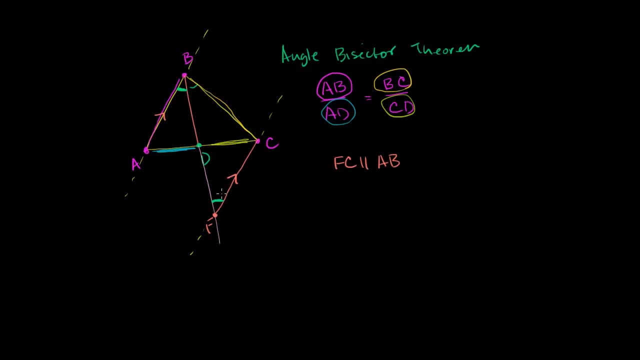 Alternate interior angles, which we've talked a lot about when we first talked about angles with transversals and all of that. So these two angles are going to be the same, But this angle and this angle are also going to be the same, because this angle and that angle 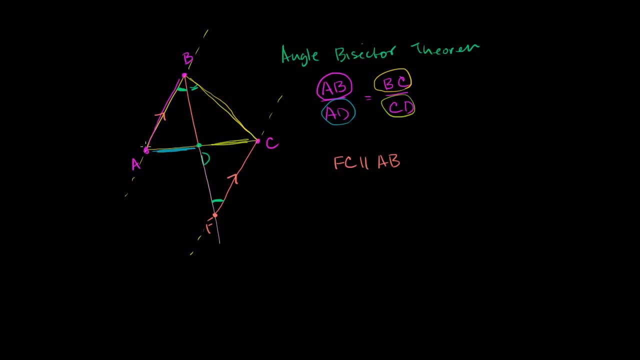 are the same. This is a bisector. Because this is a bisector, we know that angle ABD is the same as angle DBC. So whatever this angle is, that angle is, and so is this angle, And that gives us some kind of an interesting result. 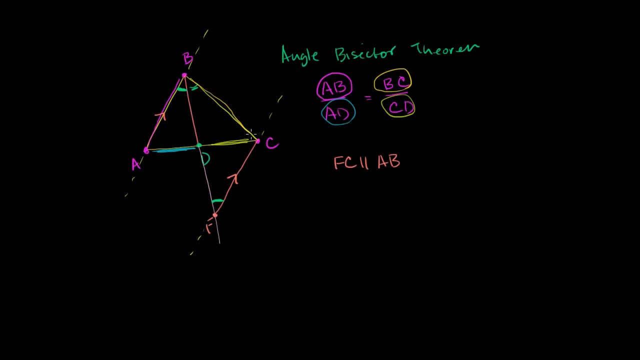 Because here we have a situation, A situation where, if you look at this larger triangle, BFC, we have two base angles that are the same, which means this must be an isosceles triangle. So BC must be the same as FC. 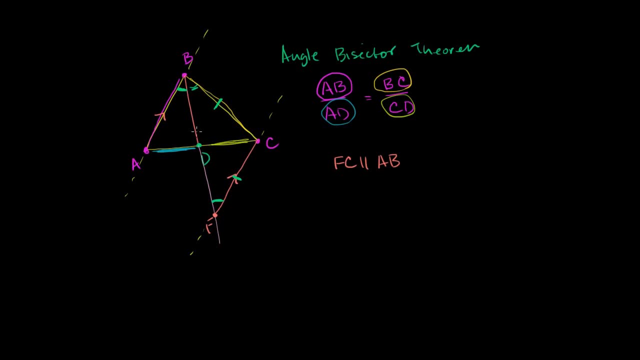 So BC must be the same as FC. So that was kind of cool. We just used the transversal and the alternate interior angles to show that these are isosceles and that BC and FC are the same thing, And that could be useful, because we know that we have a feeling that this 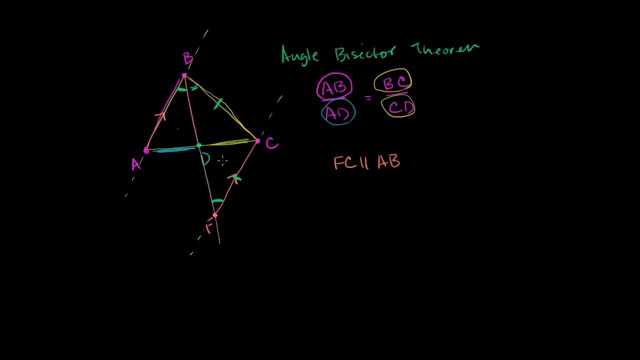 triangle and this triangle are going to be similar. We haven't proven it yet, But how will that help us get something about BC up here? But we just showed that BC and FC are the same thing, So this is going to be the same thing if we want to prove it. 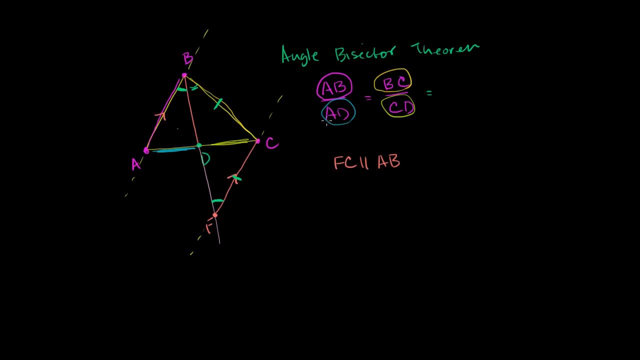 If we can prove that FC, the ratio of AB to AD, is the same thing as the ratio of FC to CD, we're going to be there Because BC- we just showed- is equal to FC. But let's not start with the theorem. 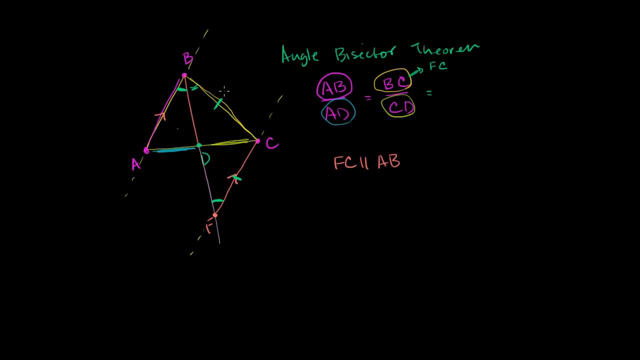 Let's actually get to the theorem. So FC is, parallel to AB, able to set up this one isosceles triangle. so these sides are congruent. Now let's look at some of the other angles here and make ourselves feel good about it. 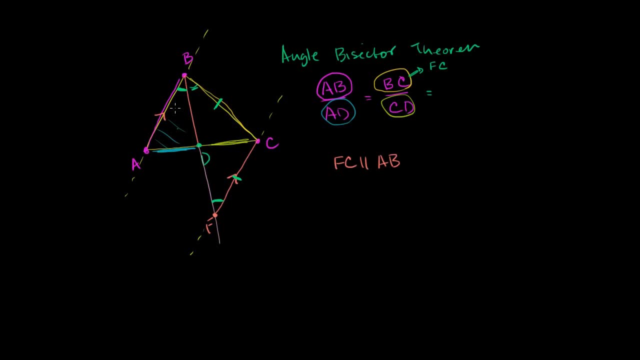 Well, if we look at triangle ABD- so this triangle right over here- and triangle FDC, we already established that they have one set of angles that are the same, And then they also both- ABD has this angle right over here. 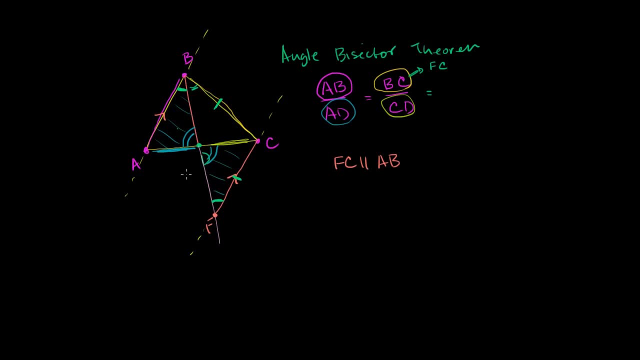 which is a vertical angle, with this one over here. So they're congruent And we know, if two triangles have two angles that are the same, Actually the third one is going to be the same as well, Or you could say by the angle-angle similarity. 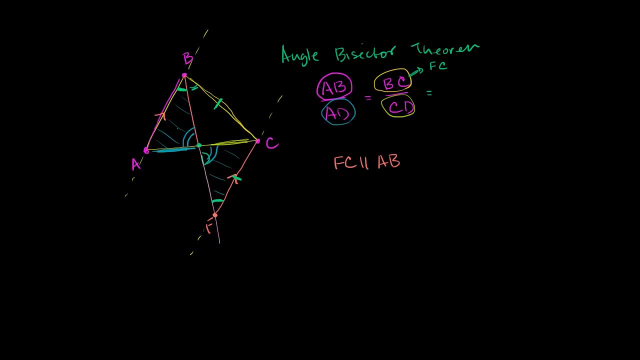 postulate these two triangles are similar, So let me write that down. You want to make sure you get the corresponding sides right. We now know by angle-angle- and I'm going to start at the green angle- that triangle B and then the blue angle, BDA, is similar to triangle. 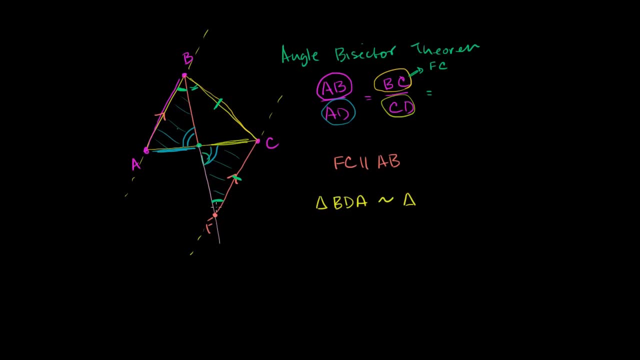 So, once again, let's start with the green angle, F, Then you go to the blue angle, FDC, And here we want to eventually get to the angle bisector theorem. So we want to look at the ratio between AB and AD. 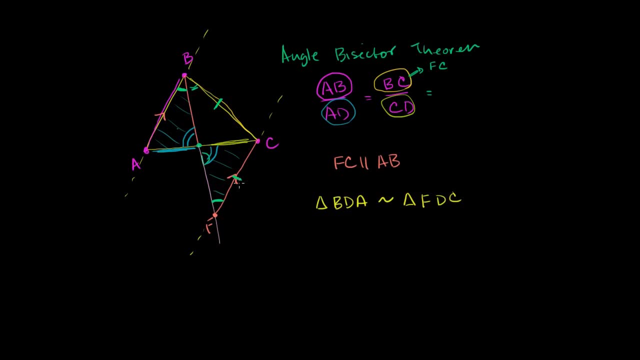 Similar triangles. either you could find the ratio between corresponding sides are going to be the same on similar triangles, Or you could find the ratio between two sides of a similar triangle and compare them to the ratio of the same two corresponding sides on the other similar triangle.